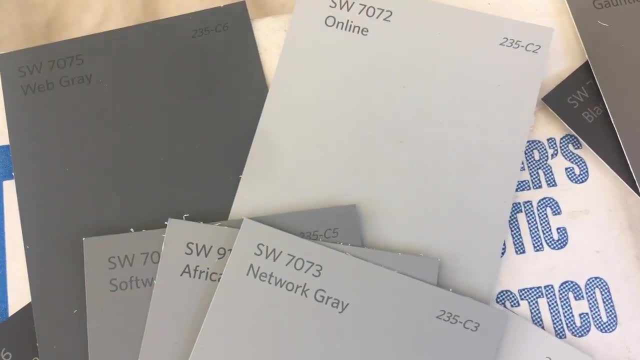 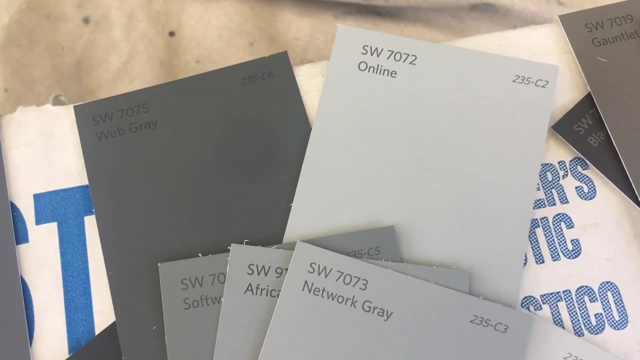 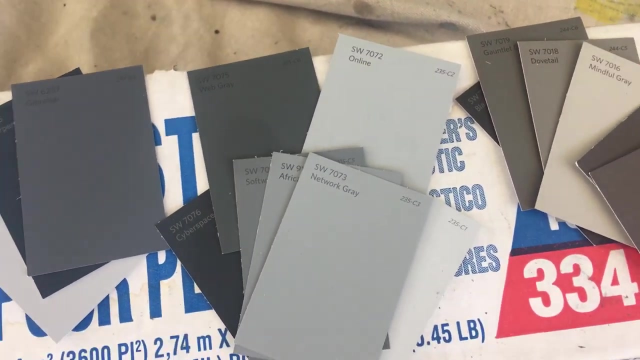 Welcome and thank you very much for watching another Christian Painters YouTube video, This one featuring exterior paint colors. It's gonna be a lot of fun. See. these are our colors we're working with here Online and web gray. I have these other sample paint chips here because I want you to be able. 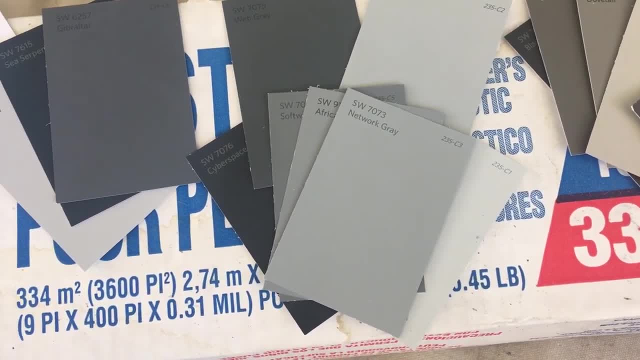 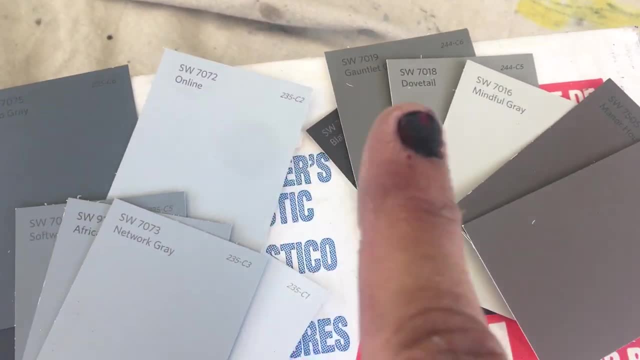 to see that there is a gray that is bluer than the gray we're working with and there's a gray that is mauve-ier, Got a little more of a red mauve hue to it. These colors look fantastic on some homes with the existing brick and powder. 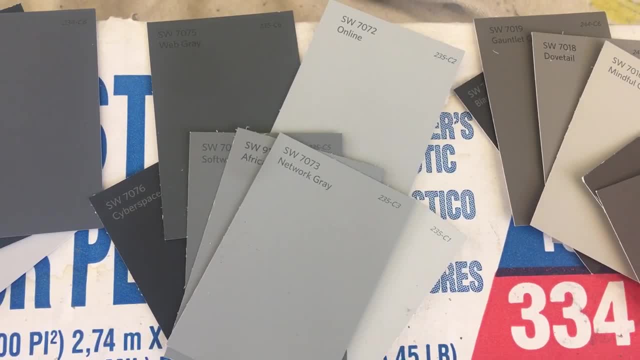 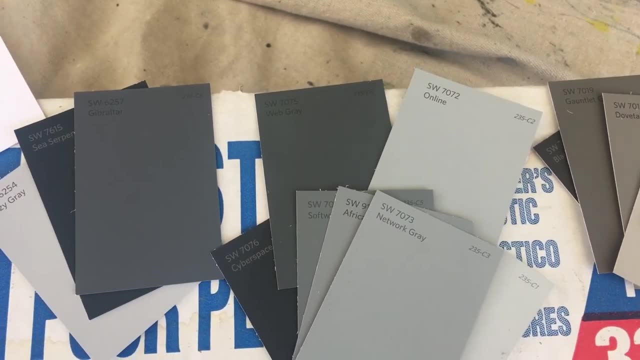 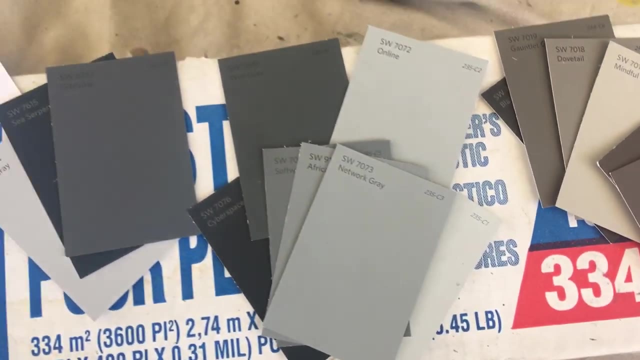 coating, but this is a lovely home in the Arlington Heights neighborhood and it needs just a little bit of pop. We've got some red cedar shingle on the front of the house and with this dark web- gray and online on the rest of the house, there's really a nice. 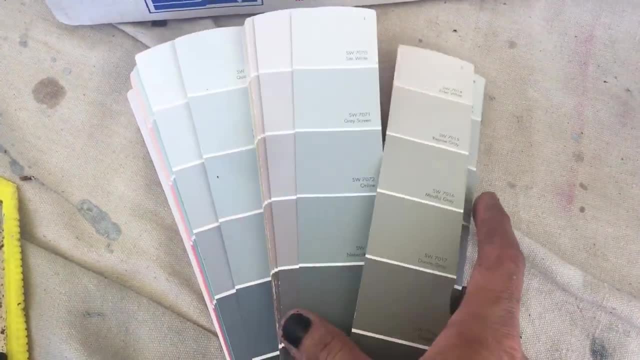 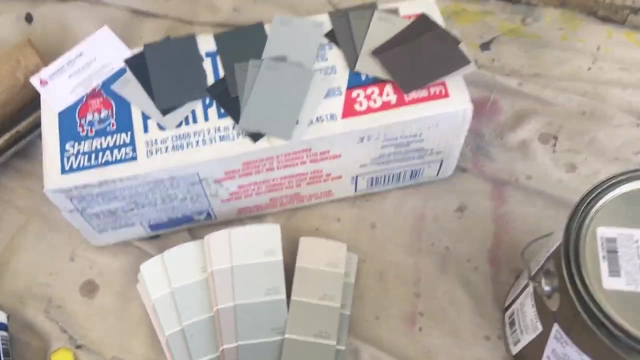 pop with those colors. Here's the old Sherwin-Williams fan deck. I just want you to see there are bluer grays and, yes, happy Halloween. This is Halloween weekend. Right here I happen to have some of our product Sherwin-Williams exterior. 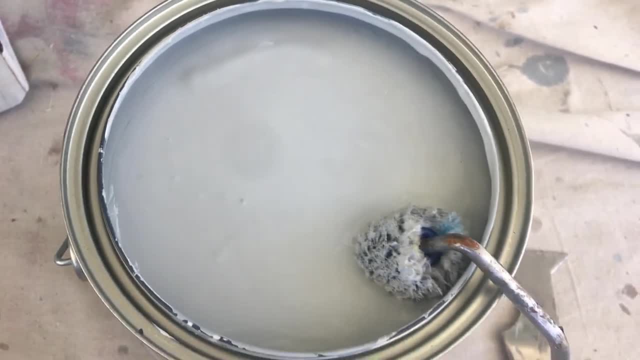 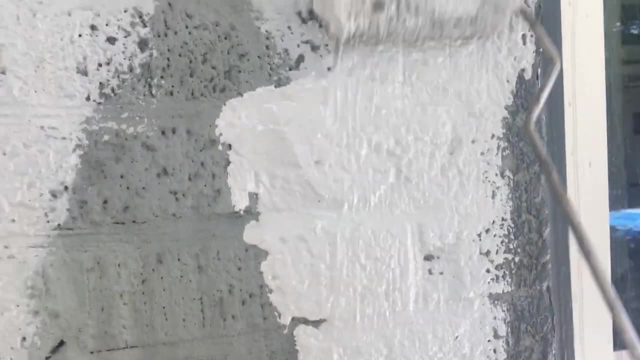 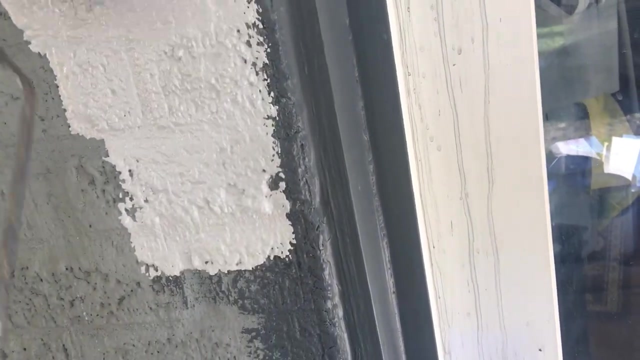 super paint. Take this lid right off. Look there it is. That's our color online and I've already put a little up here. I'm gonna put there. you go a little more right up here next to the gray. I'll show it from this angle so you can see that dark gray which is web gray. 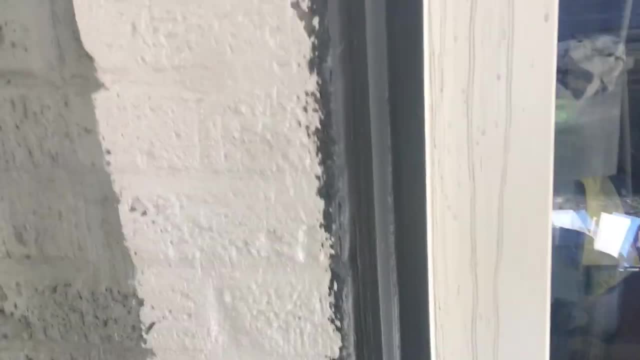 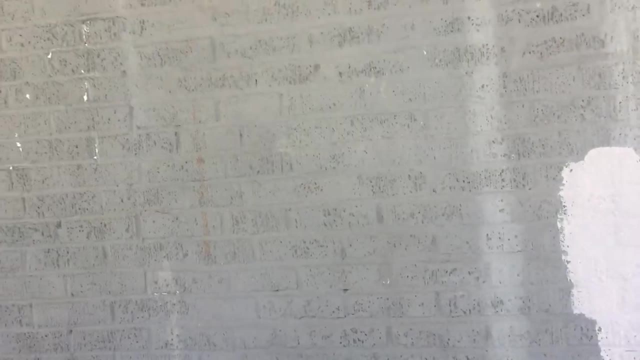 right there next to the online and see how that's going to look on the house, As I show you the back of the house that is getting ready to be painted. I've already painted the whole house. all the blue, dark gray. There you go, all the dark gray. 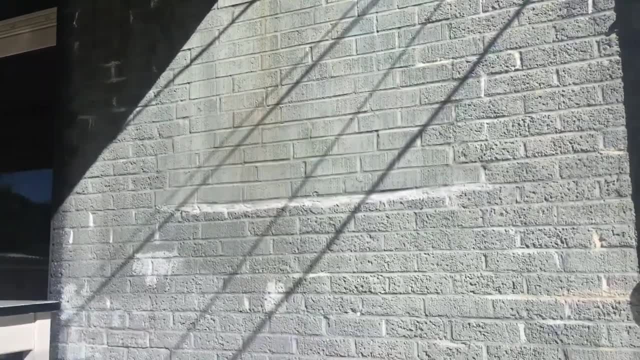 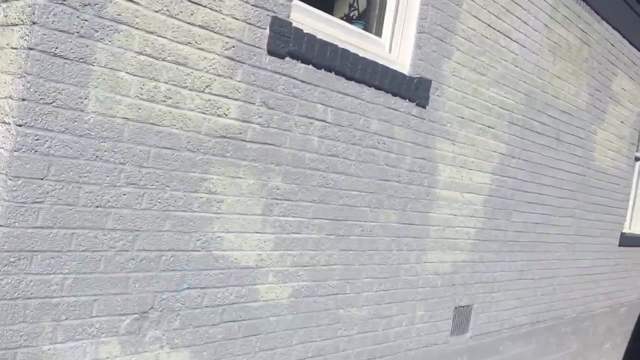 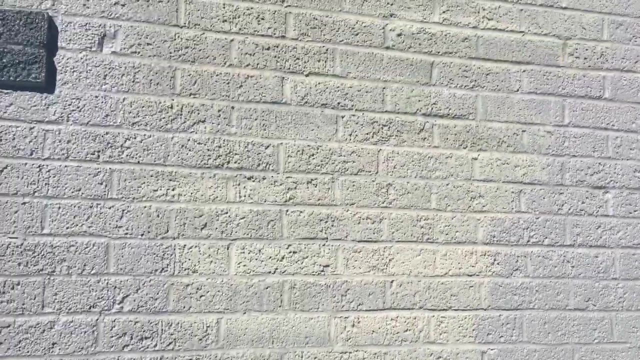 is done up top. All the stucco is done up top. but you can see where all of this brick has been caught and primed. it is prepped and ready for paint, kind of like. this is: all of this is painted through here and on down that direction. but I've got a couple of spots here. you can see the old. 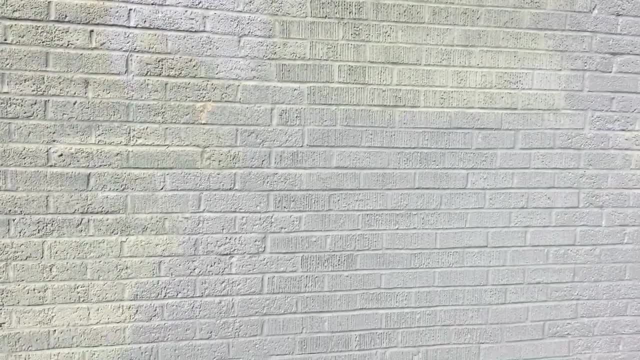 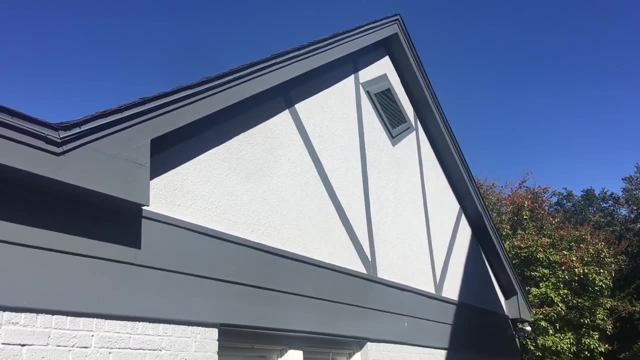 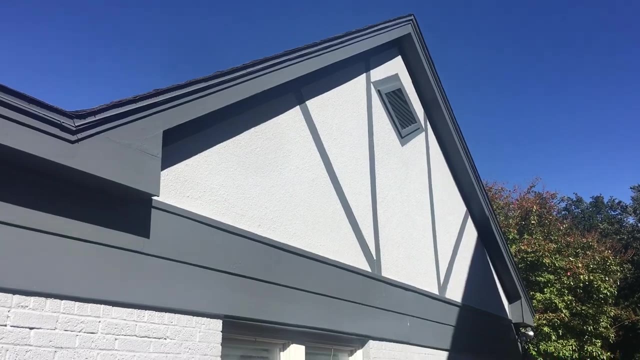 paint. so that'll be getting painted today as well. I want to show you the top of this house, where the colors really come together and pop, and then I'll run you around the front. so those are our colors: web gray and then the lighter color is the online. so that's what our house looks like.